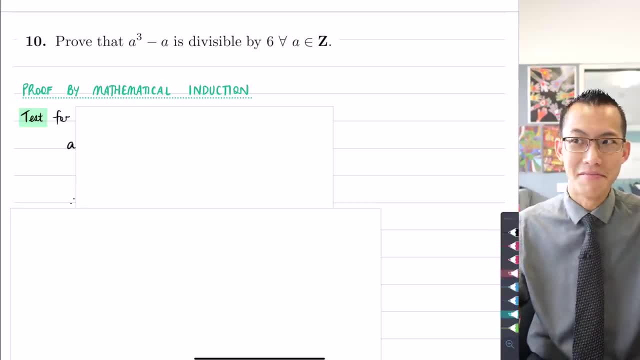 start counting up one, two, three, four, five, six. you have missed like half of the integers, all of the negative ones. right, You could start from some number earlier on, like negative one or negative two or negative three, but you still run up against this fact, that induction as we. 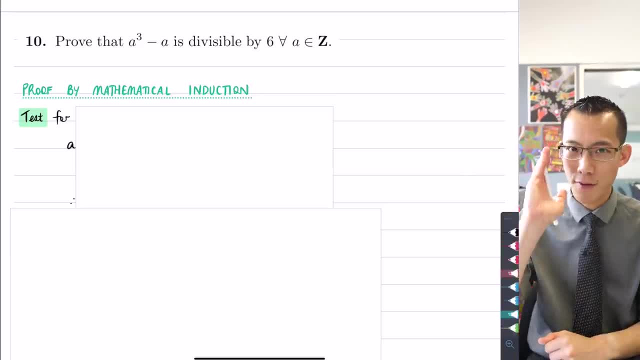 have learnt. it is a mono-directional process, So it's always going to start from one value- the base case- and then keep on going in one direction. Now, this is not going to work by not an impossible barrier to overcome, If you think back to when we proved de Moivre's theorem. 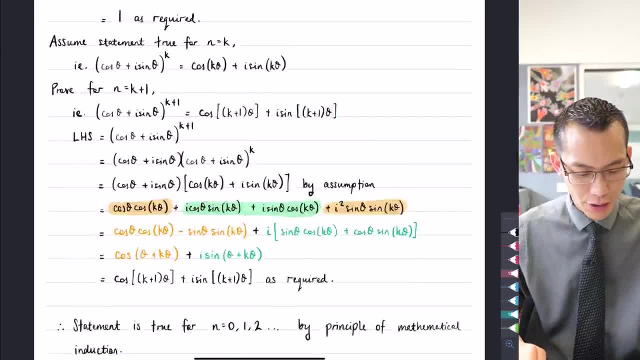 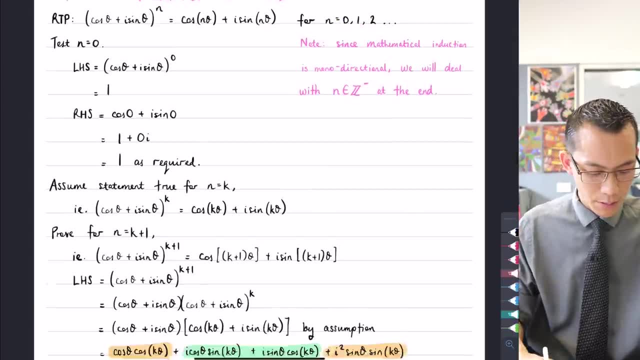 we could actually do that by mathematical induction And I actually showed. if you start off by saying: look, let's have this statement here and consider it for 0,, 1, and 2,, it becomes, and so on, it becomes a fairly straightforward use of some trigonometric identities and some 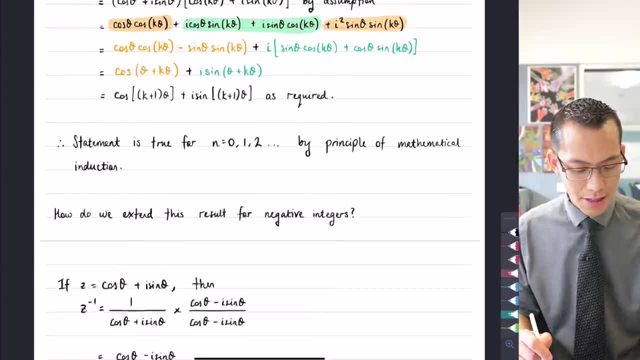 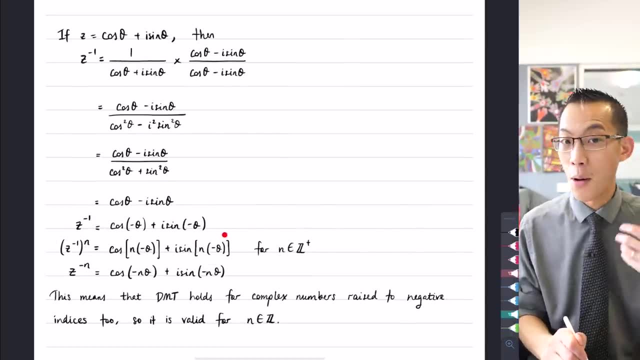 rearrangement. You can prove this, and then you just need to cover the negative integers. So you need to use some other trigonometric identities to handle that. You use the result that we just proved for positive values of n and then off you go. It's fine for the negative values too. 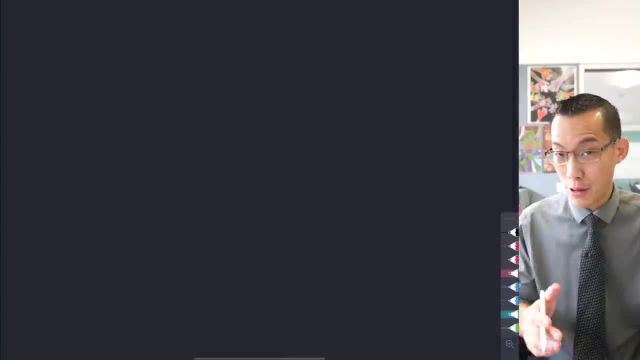 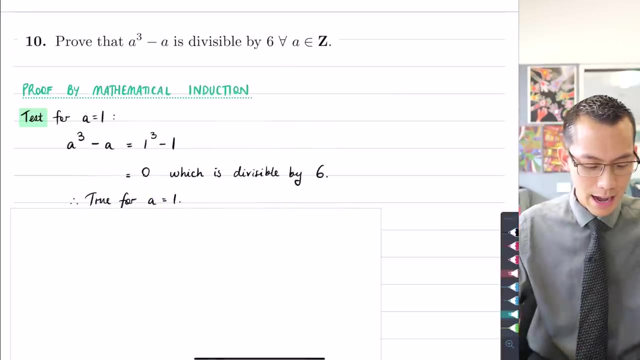 But it's worth keeping in mind that this is not just going to be if we use mathematical induction, it's not just going to be a straight proof. We're going to have to handle half of the cases. So here you can see me choosing, you know, 1 as my first value, and then I'm going to have to. 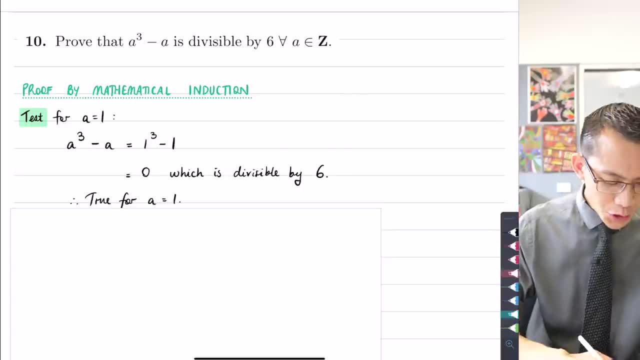 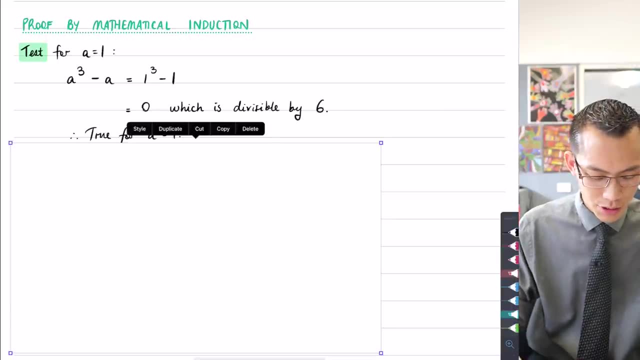 do all that work and consider the negatives as well. So first snag, sort of address. I haven't solved it, but I know it's there. My second snag comes after I do the assumption step. You can see I'm just going to assume that this is true for some arbitrary value of a 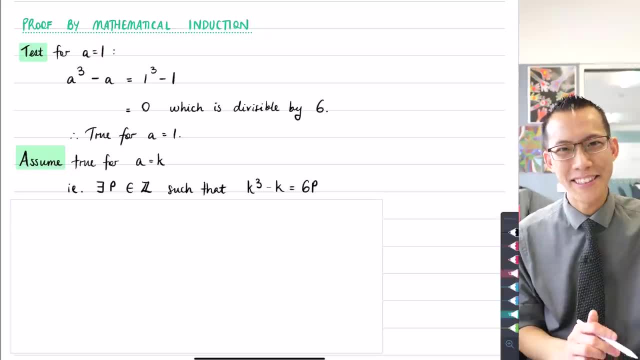 and what I can say is using some of the notation that we have learned recently. in The Nature of Proof, there exists some value of p where p is one of the integers, such that k cubed minus k is 6 times p. So what I'm saying here is k cubed minus k is going to be some. 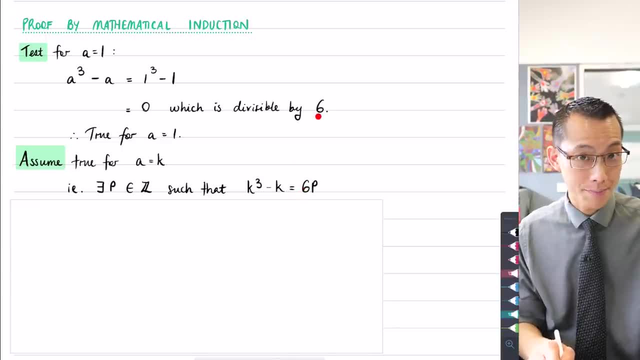 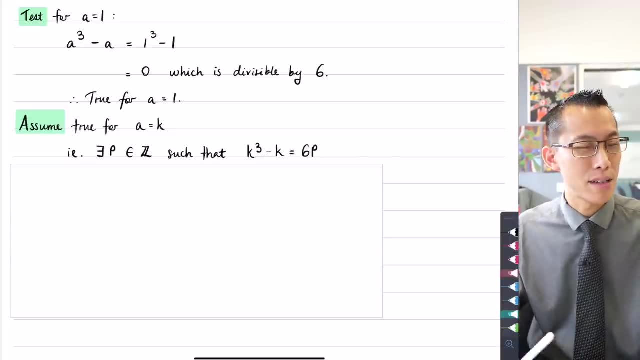 multiple of 6, which is analogous to the value of a. So what I'm saying here is I'm going to equivalent to saying it's divisible by 6.. And we know the assumption step isn't a whole lot of work. It's the proof step, not for k, but for k plus 1, where the real rubber hits the road. 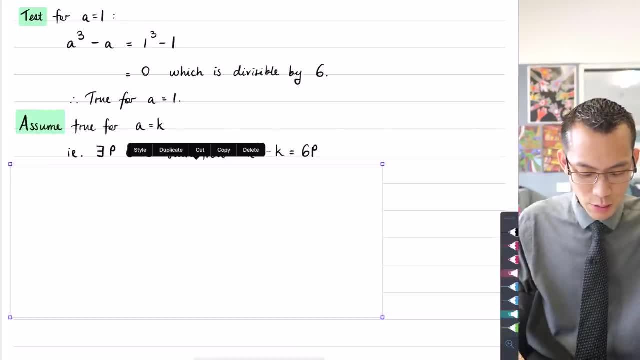 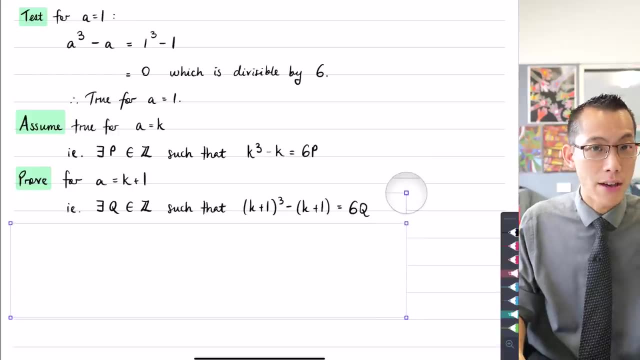 And this is where we hit our second major snag. You can see what happens when we just say: well, let's just see what happens for k plus 1. We go ahead, substitute it in. I'm going to say there exists some value, q, which is also an integer, which is going to give me my new multiple of 6.. 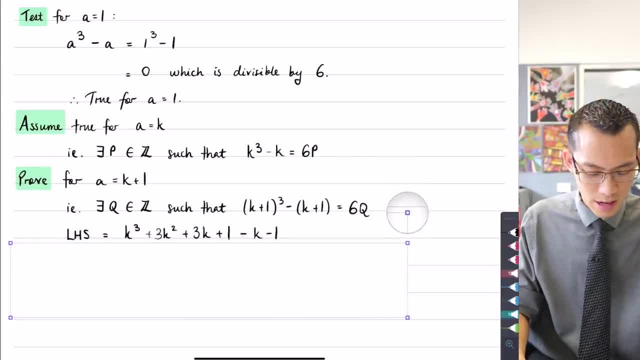 And then I do my substitution into the left-hand side and say: well, what's going to happen here Now? those of you who remember mathematical induction will recall that what you want to do here is try and twist and turn this algebraically. 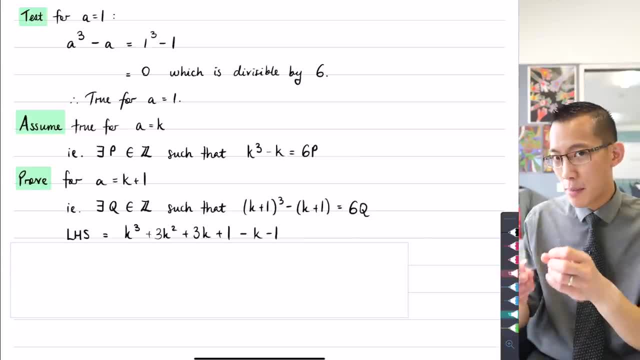 in order to make the inductive hypothesis the assumption, to make it sort of appear, and then you can do a substitution and then, hopefully, things fall out in the wash and you arrive. if you're starting on the left-hand side, you arrive on the right-hand side. 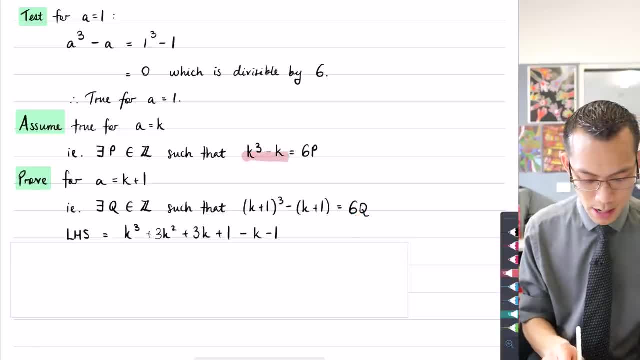 Now, when I have a look at my inductive hypothesis which is up here: k cubed minus k equals 6p. you can actually already see k cubed and minus k in the left-hand side of my equation here, right. 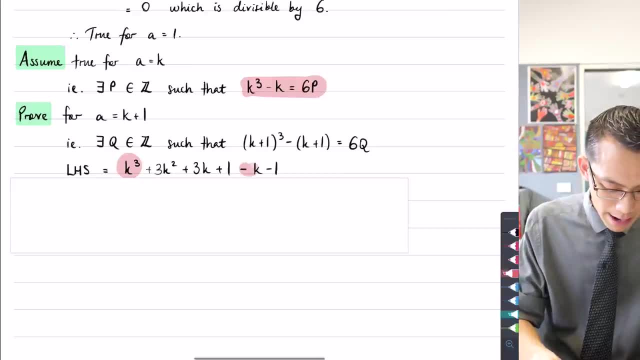 Expression I should say: This is the k cubed and here is the minus k, So I could just substitute those for 6p by assumption. Then there's a bit of other simplifying as well. that will happen. So let's watch what happens. what takes place when I do that substitution. You can see I've. 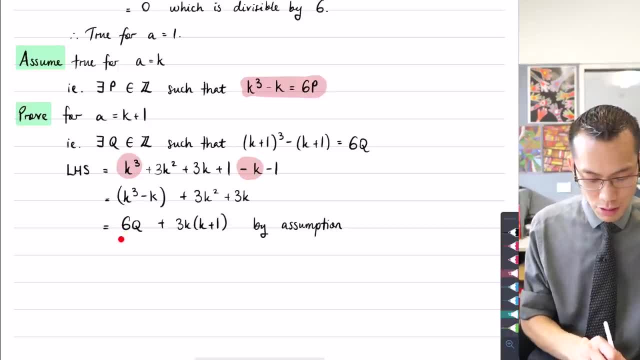 brought this k cubed minus k out the front. I've substituted for 6q. I notice my plus and my minus 1 have canceled with each other, leaving me with 6q, So I'm going to substitute those for 6q. 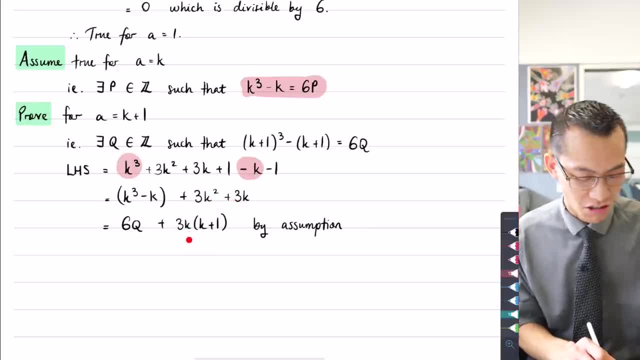 I'm going to do this and then I have done this factorization because I notice the 3k can come out the front. Now, at this point you pause because you think: great, I want to prove that this is equal to. actually, that should be a 6p, not a 6q. Let's fix that up. I've got this. 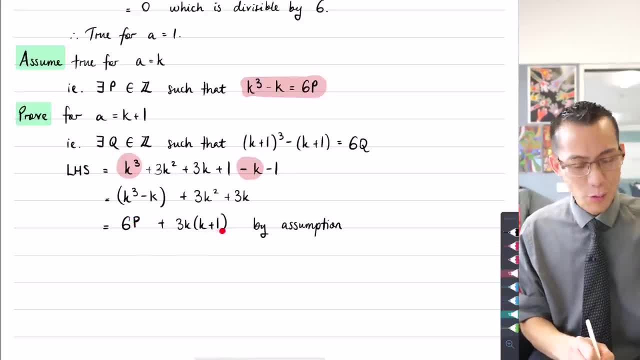 part at the front. This part is divisible by 6.. Great, Then I have to deal with this. What do I do with this set of terms over here? Now, the short answer is probably: in this scheme, the most efficient way to go about this is not to do this. I'm going to do this. I'm going to do this. 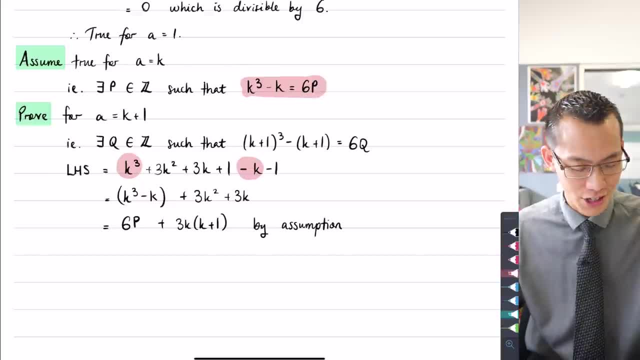 Not very efficient at all. I have to kind of start a whole new proof by induction to handle this part of things. Prove that it is divisible by 6, and then I can do a substitution. So I've got this multiple of 6, another multiple of 6, and then everything will be fine And it's. 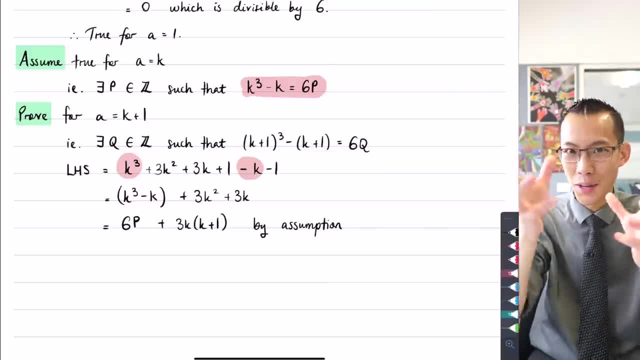 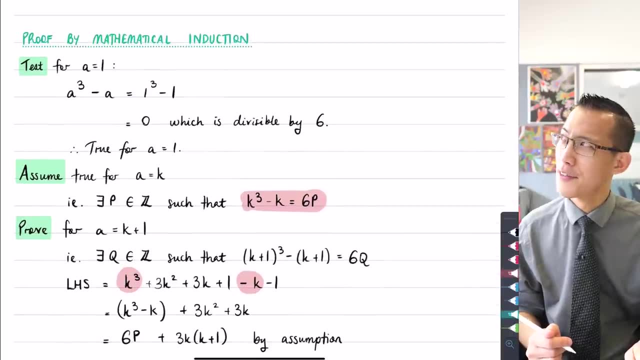 worth merging. Sometimes you have to do that. Sometimes you have sort of a babushka doll situation. It feels like you're differentiating by the chain rule. It's like, oh, not function of a function, It's mathematical induction of a mathematical induction. This is the second. 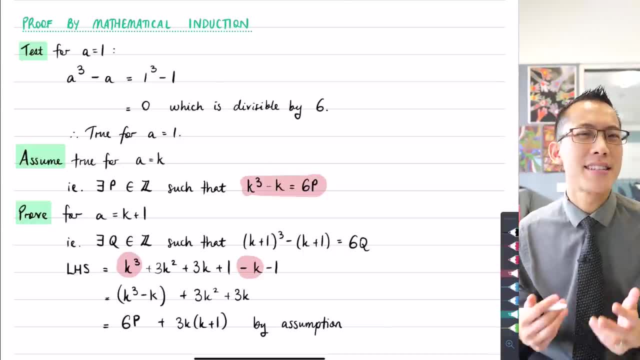 snag that I was talking about Can work, but certainly doesn't seem elegant right. Is there another way that we can go about this? The answer is yes. We're going to have to improve- sort of not improve. We're going to have to employ some deductive logic that we're not used to using in. 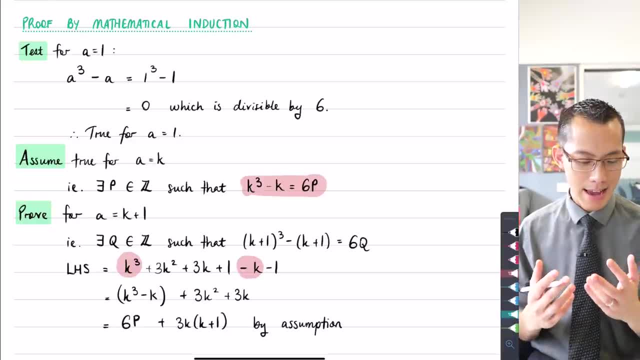 the context of number theory, but it's going to be much more elegant, even though it might in the end, end up being sort of a similar amount of working. But I think that the flow of the logic will be much clearer. So let's rewind, Let's go back to treating this question from the 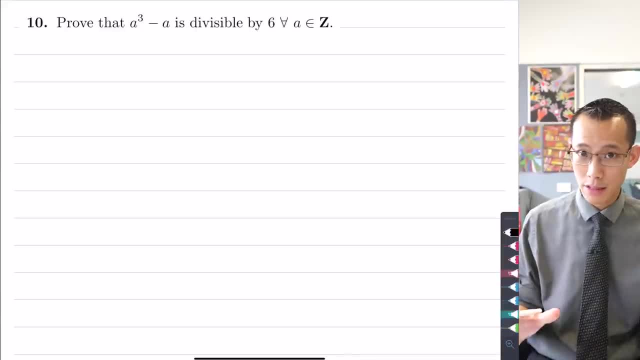 beginning. How can we go about proving this without resorting to induction? What I'm going to do first is I'm just going to take this expression here, a cubed minus a, and I'm going to see if I can gain any insight from it by manipulating it algebraically. So what I'm 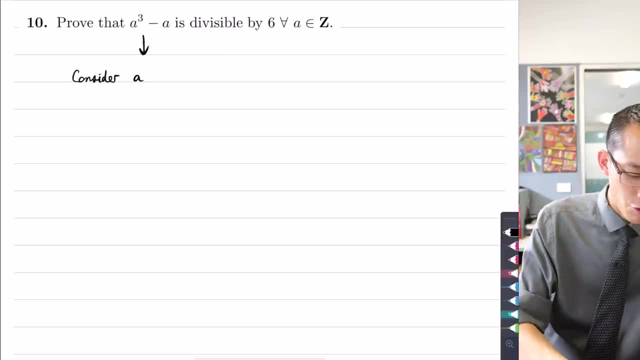 going to do is: I'm considering a cubed minus a. Now what can I do with this? The most obvious thing that jumps out at you is say: well, I can factorize this. In fact, I can factorize it a couple of times. I can first. 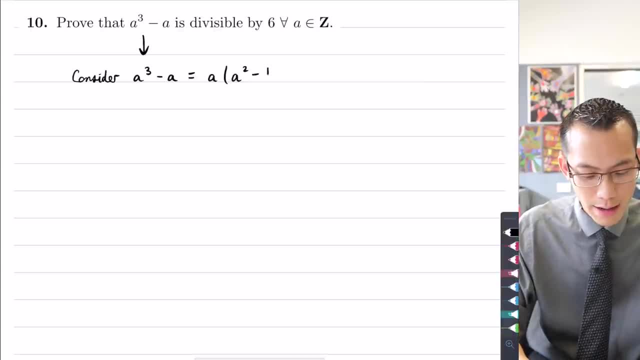 take out that common factor of a, That leaves me with a squared minus one. And then you think: fantastic, I have differences, squares here. So I've got a outside of a minus one, a plus one, And at this point it's all factorized. And you might think: well, what can I do with this? 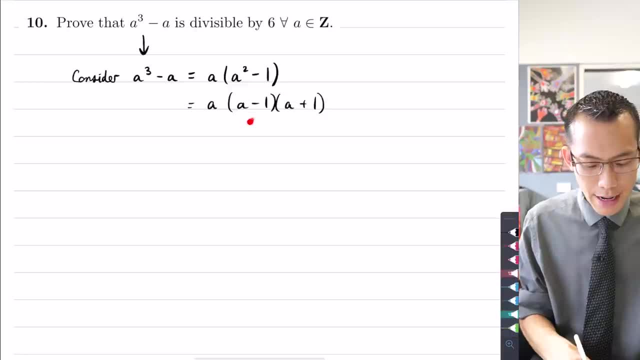 What I want you to notice is that what you have is a product of three different numbers, but they're not just three random numbers: A and a minus one and a plus one. they're actually connected, They're related, in that, if I put them in this order- a minus one and then a and then a plus one- what you can see 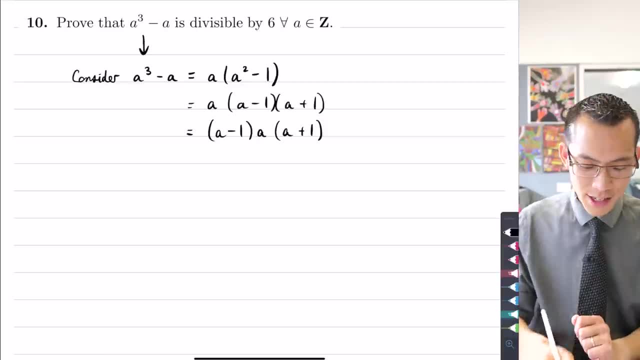 here is. I actually have three consecutive integers. You've got one number here in the middle, a number one less and a number one more. So I've got three integers in a row here. Now, this is important. It's so important that I'm going to write it down. I'm going 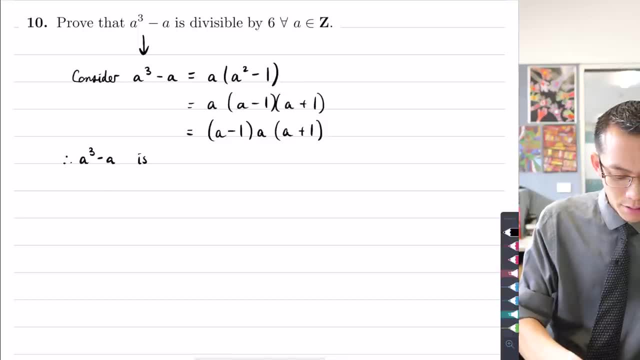 to say, therefore, a cubed minus a. So I've got three integers in a row here And I'm going to say a cubed minus a is the product of three consecutive integers. Now, at this point, three consecutive integers. At this point I need to think before I make any further. 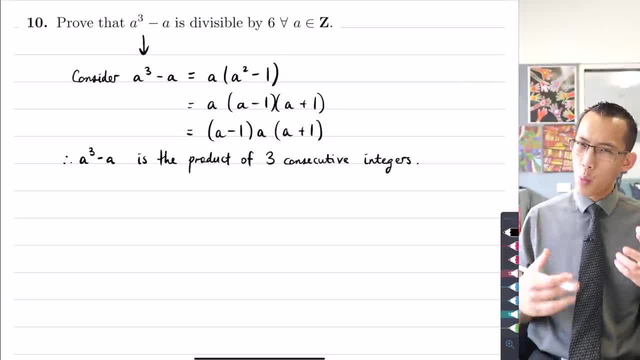 algebraic marks on my page. how can I use this property- The fact that a cubed minus a can be written as the product of three consecutive integers. how can I use this to construct a proof? Here's how it's going to go about. I want to prove that this is divisible by 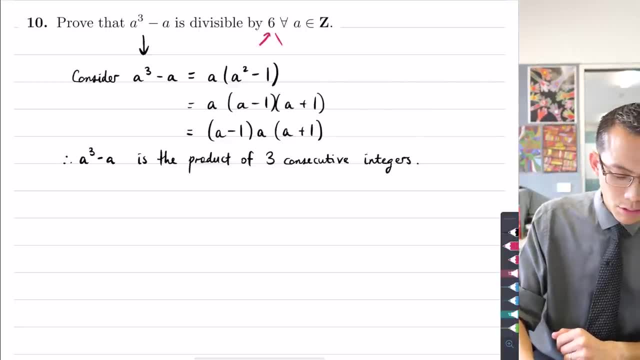 six. Now, six itself, I can break into two component pieces because six is a composite number. If you were to factorize six, it would break into two times three. Now what that means is if a number is divisible by six, that implies it's also divisible by two because it's even. 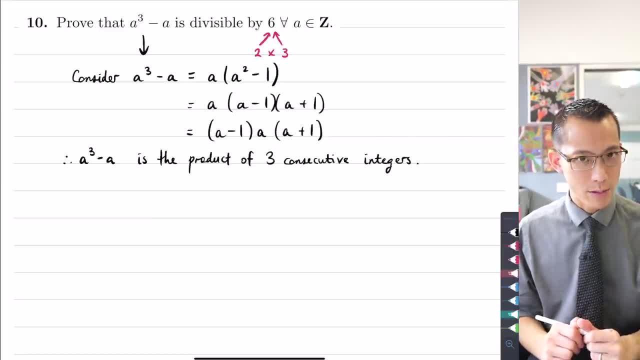 and it's also going to be divisible by three. It should be a multiple of three as well. So therefore, if I can prove this in the opposite direction- because these are equivalent statements- If you're divisible by six, then it must be divisible by three. So therefore, if I can, 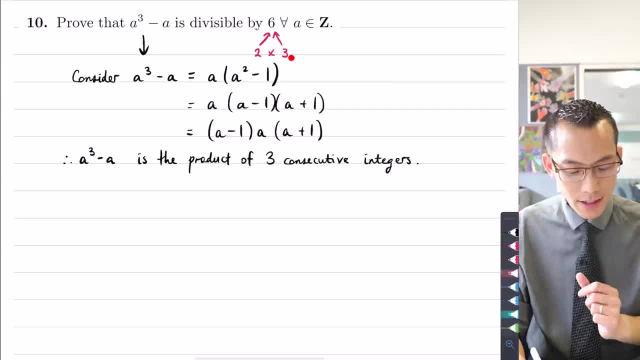 prove this in the opposite direction, because these are equivalent statements. if you're divisible by three, it must be true that you're divisible by two and three, but if you're divisible by two and three, you must be divisible by six. If I can prove this sort, 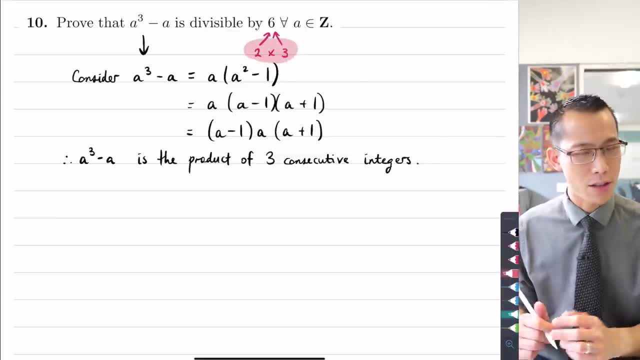 of pair of results, then I have proved the initial result that I set out to actually prove. So that's my roadmap through this question. If I can prove this is by two as divisible by three, I'm good to go Now. if you just think about this and maybe an example, 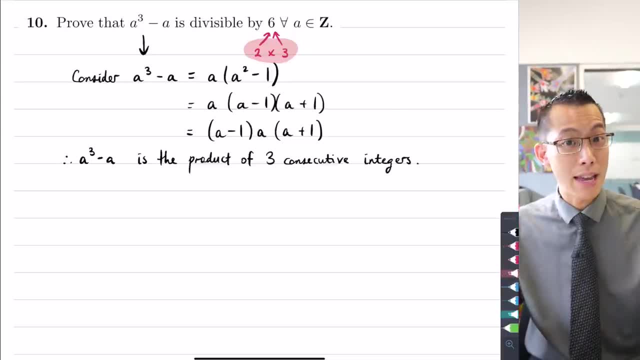 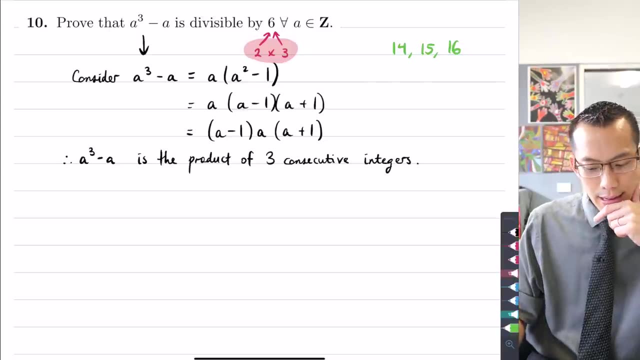 would be instructive here If you thought of three consecutive integers, any three consecutive integers like, say- I don't know- 14,, 15,, 16.. What you see here is, if you pick any three consecutive integers, at least one of them is going to be even. In this case, I've got 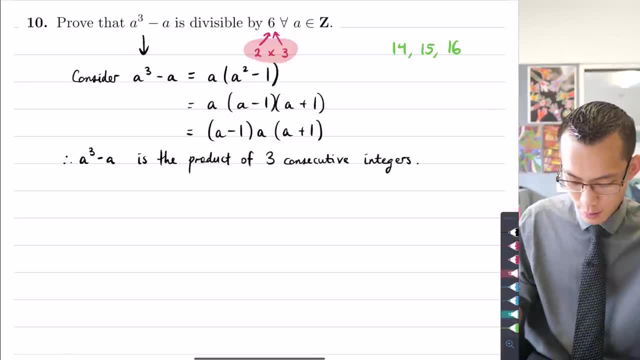 14 and 16.. They're both even right, But if I went along to the next one, let's suppose I scrapped 14 and I considered the next one. you can see here, even though I don't have 14 anymore, 16 is still there, So you're always going to have at least one number, that's. 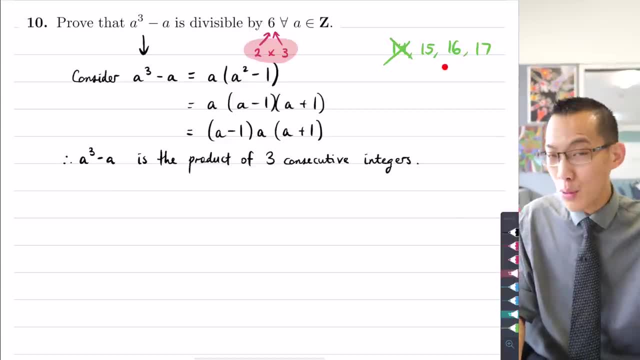 a multiple of two. And because you've got three numbers, you also will always have at least one number that's a multiple of two. And because you've got three numbers, you also will always have at least one number that's a multiple of three. In this case, it's 15.. If I were to